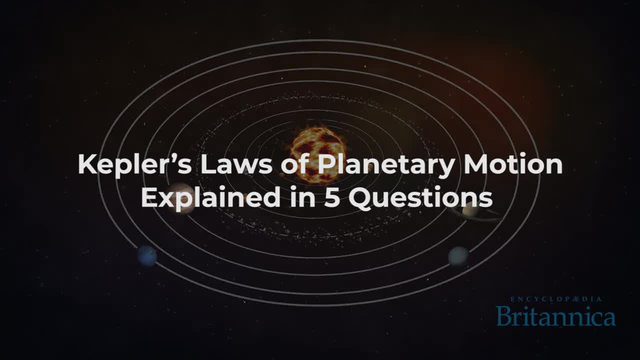 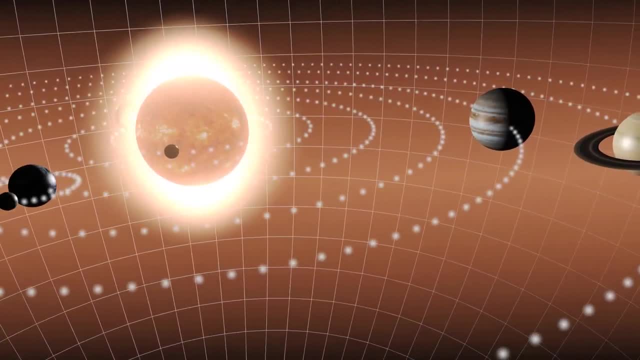 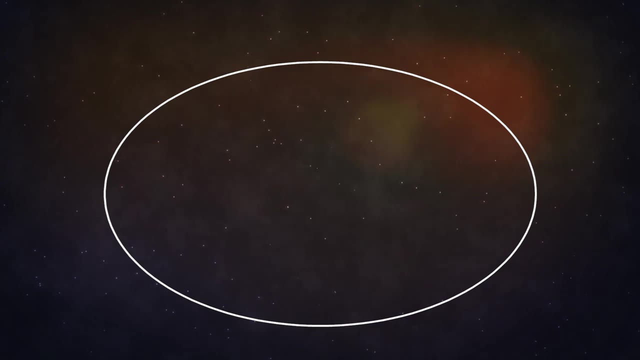 Kepler's first law of planetary motion states that all planets move about the Sun in elliptical orbits, having the Sun as one of the foci. But what does that actually mean? Well, an ellipse is a shape that resembles a kind of squashed circle. Its foci are two points within. 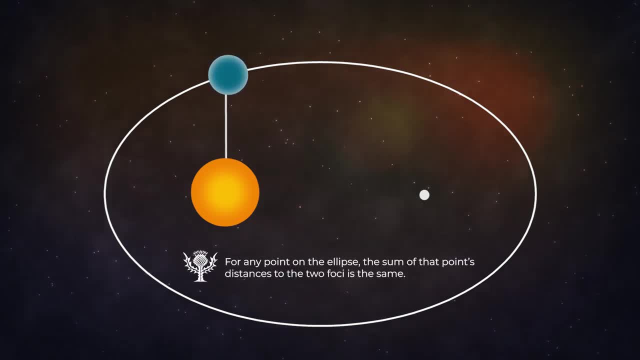 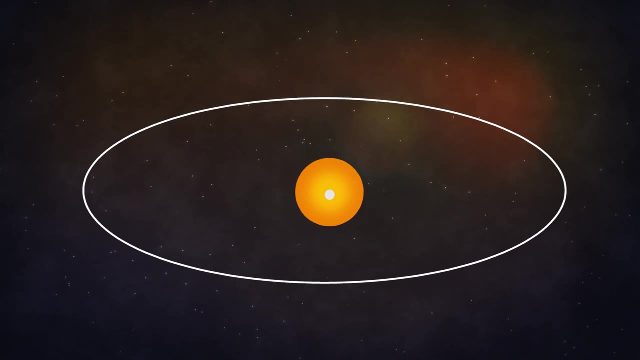 the ellipse that describe its shape. For any point on the ellipse, the sum of that point's distances to the two foci is the same. The further apart the foci are, the more squashed the ellipse is. If the foci become so close that they are only one focus, you just have. 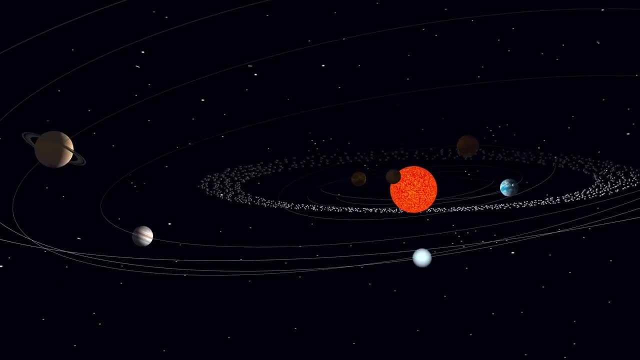 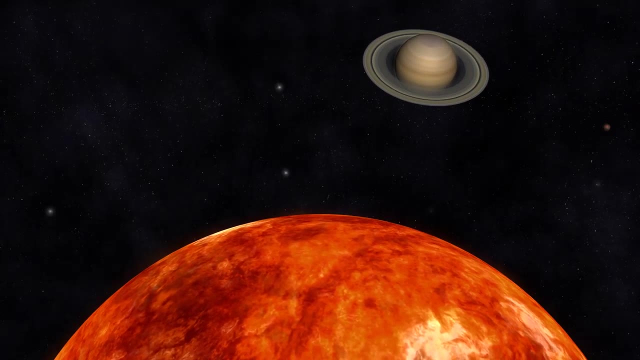 a circle. In reality, orbits are never perfectly circular, But we do know that the Sun will always be one of the foci of the elliptical path of an orbit. Knowing that the Sun is a focus of the planet's orbit can tell us a lot about the shape of that orbit. 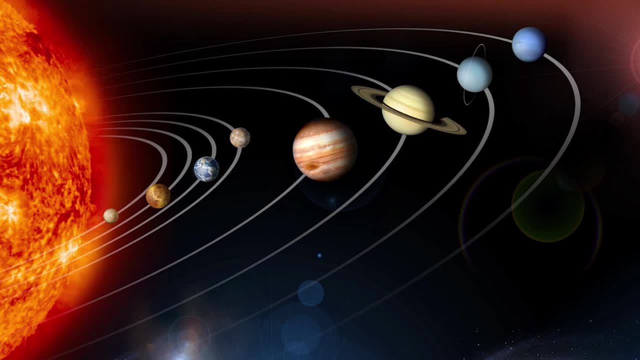 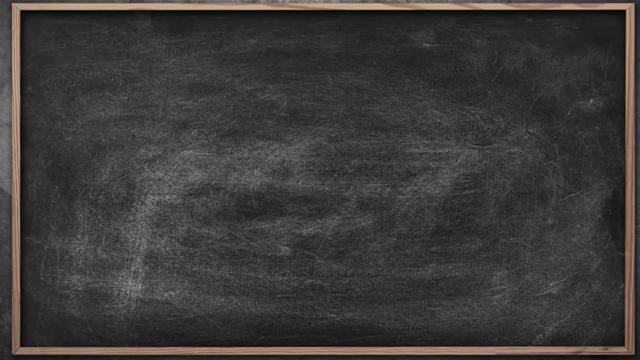 Kepler tells us that orbits are ellipses, which are like circles, with some added eccentricity. But what is eccentricity? How do you figure it out? Eccentricity measures how flattened an ellipse is compared to a circle. We calculate it using 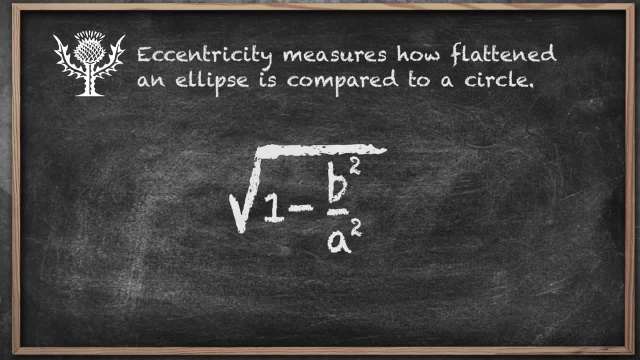 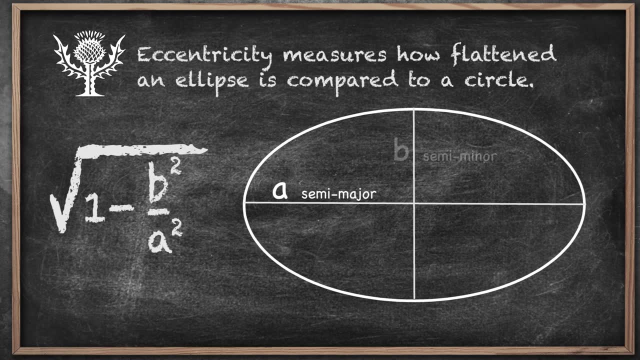 this equation. So what does that mean? Well, a is the semi-major axis, or half the distance along the long axis of the ellipse, and b is the semi-minor axis, or half the distance along the short axis. The equation is a way to compare these axes, to describe how squashed the ellipse is. 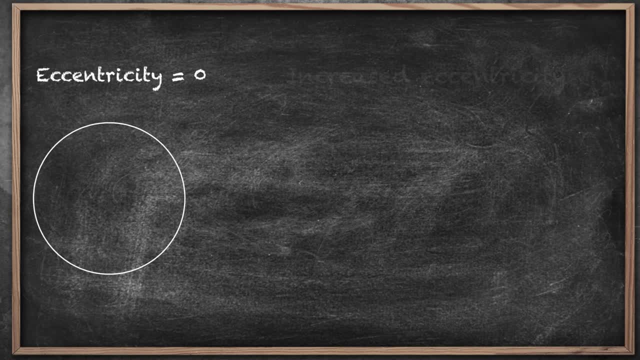 An ellipse with zero eccentricity would just be a regular old circle. As eccentricity increases, the ellipse gets flatter and flatter, until it just looks like a line. An orbit with an eccentricity greater than one is no longer an ellipse but a parabola. if e is equal to 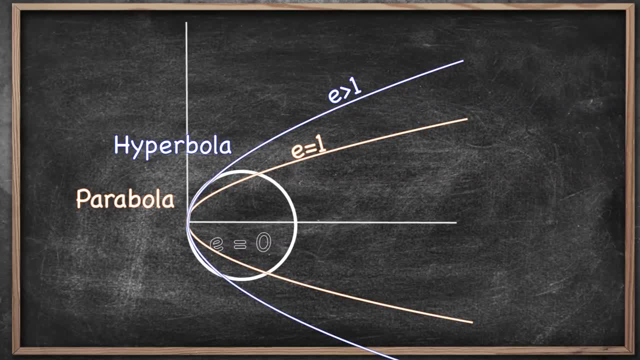 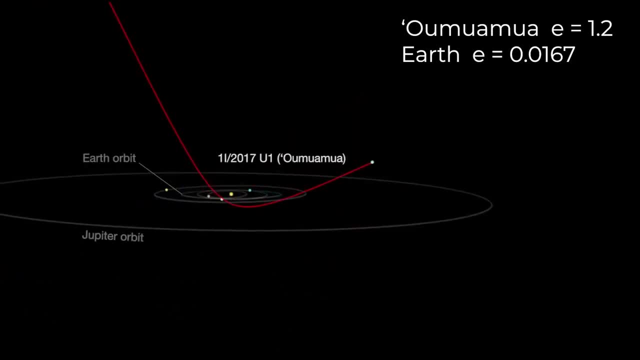 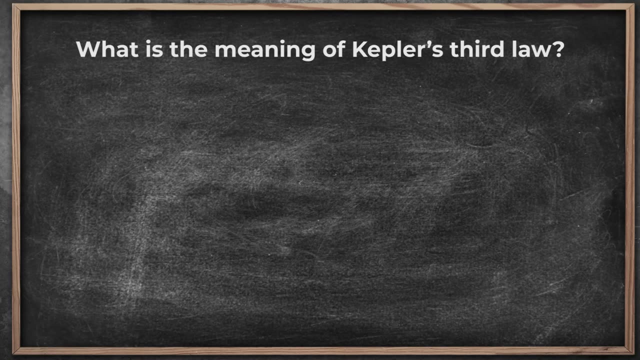 one, or a hyperbola, if e is greater than one, For example, the giveaway that Oumuamua won- the first interstellar comet was not from around here- was that its eccentricity was one point two. The eccentricity of Earth's orbit is only zero point zero. one, six, seven.